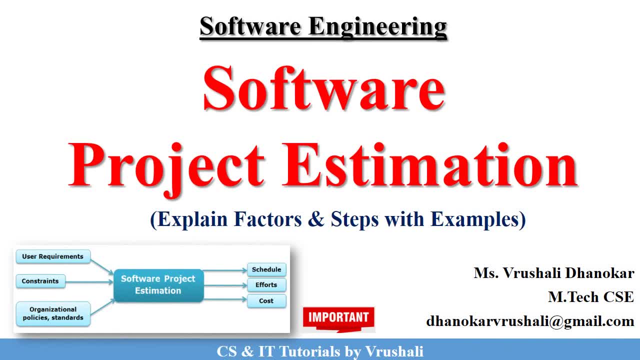 Hello everyone. this is Vrishali. In previous session we discussed about software measurements and matrix with examples. I have mentioned complete software engineering subject playlist link in below description box. Now in today's session we will discuss the next important topic, that is, software project estimation. Let's start the session. 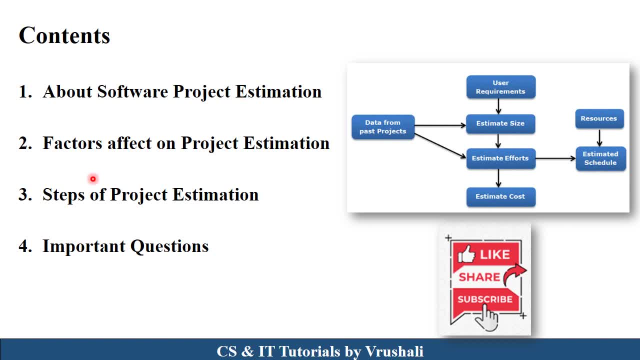 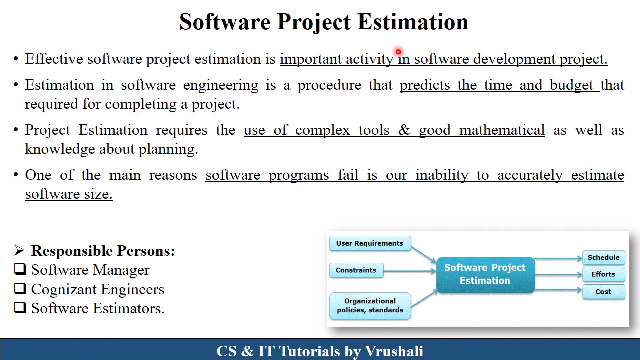 In this session we will discuss about software project estimation, their factors and steps And some important questions that have asked in previous year question paper. Let's see all these points one by one Now. the first thing is: what exactly software project estimation? See, sometime you complete software program and software project get. 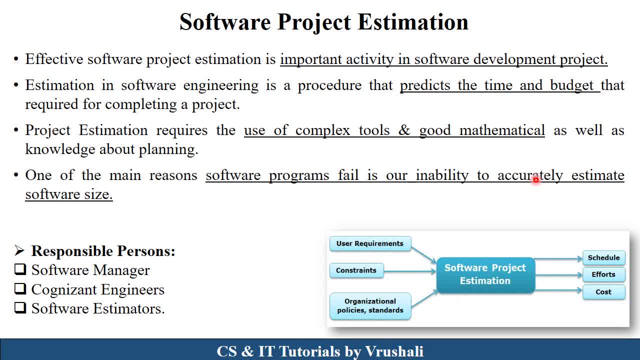 filled due to inaccurate estimation of software size and cost. For solving this type of issue, software project estimation play important role in software development project. Basically, software project estimation predict total time and budget required for completing a particular project. for that purpose, they use some complex tools and good mathematical and. 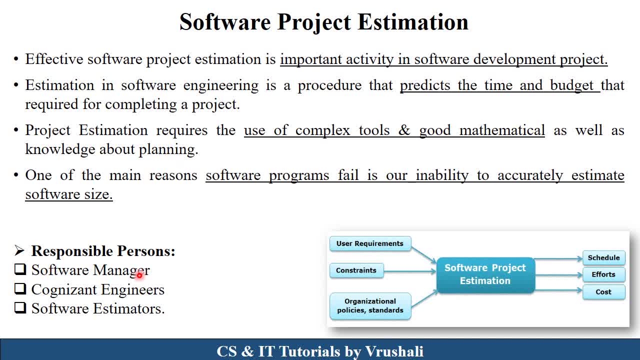 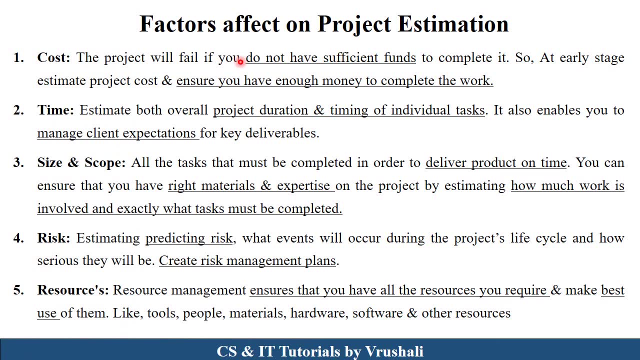 planning skill is required. there are software manager and cognizant engineer and software estimators. these are the responsible person for handling software project estimation activity in planning phase of software development life cycle. now the next topic is different factors affect on project estimation. the first important factor is cost, because the project 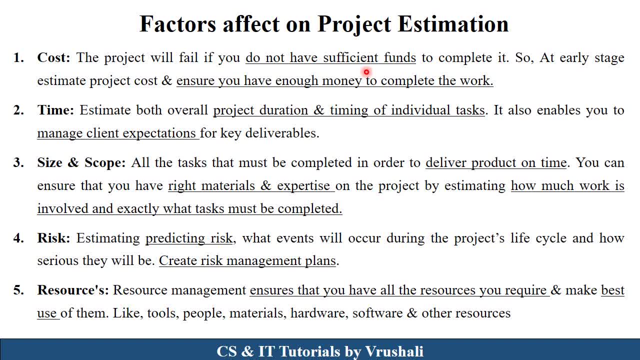 will fail if you do not have a sufficient fund. that's why project manager ensure that you have enough money to complete a particular project. they ensure all those thing at early stage of software development. the next factor is time. here project manager ensure that the complete deadline of particular project and also how much time is required to complete the project. 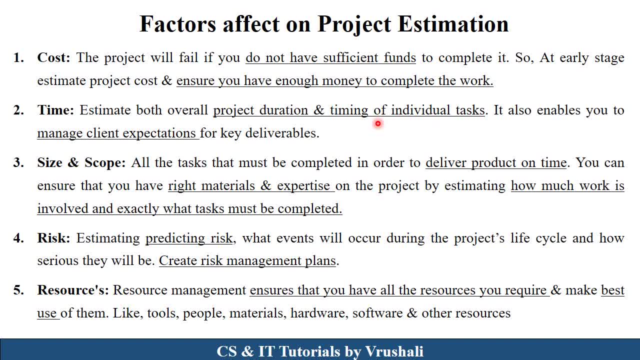 for example, in order to complete the project, you have to save a certain amount of money for removing the project. so the product will be processed in that time and the measure of time is required for performing the individual task and the end. you have to deliver a particular 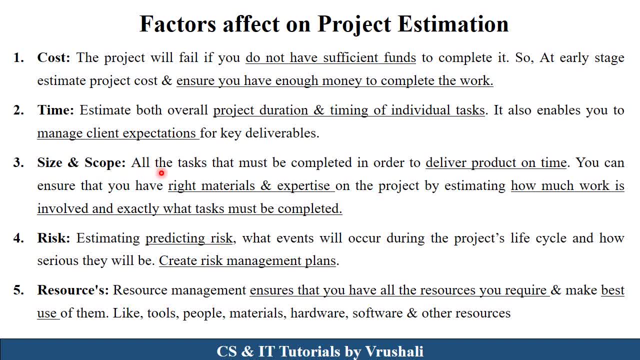 product within a deadline, within a schedule. the next factor is size and scope. here project manager decide a complete size of project and according to that they provide right material and right expertise. basically, they estimate how much work is involved and exactly what task must be completed. the next factor is risk. here project manager predict which task. 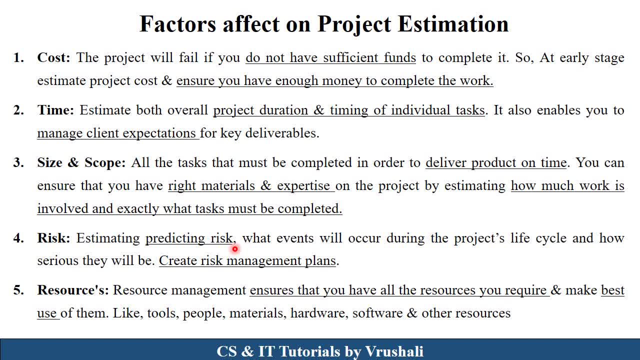 must be completed or which changes must be followed. so this is the first factor. the next factor is risk. here, project manager predict which times are needed to complete a project, that is, time is not required for of risk and problems will occur in particular project. according to that, they create risk. 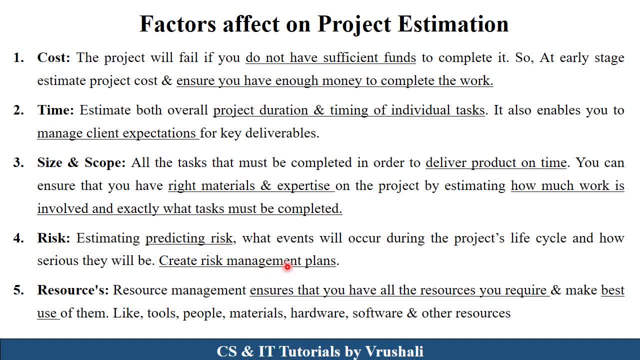 management plan. we will discuss risk management plan in detail in next session. and the last factor is resources. for developing a particular software project, resources are necessary. so project manager ensure that there are proper hardware resources, software resources or human resources are there. they provide roles and responsibility for each and every software team. so these are the different. 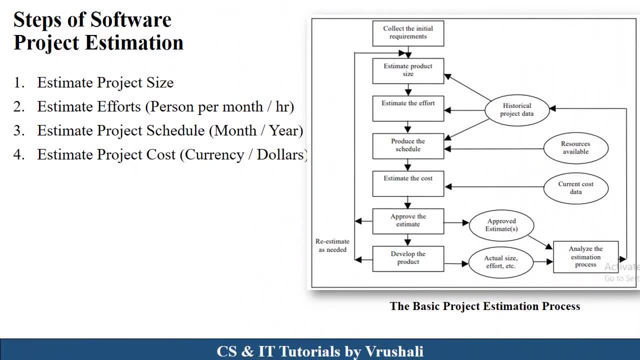 factors affect on project estimation. now the next important topic is steps of software project estimation. see here in this diagram. this is a basic project estimation process. the first thing is to collect all the initial requirements. this is a requirement gathering and analysis phase. after that, in planning phase, software estimation have start. 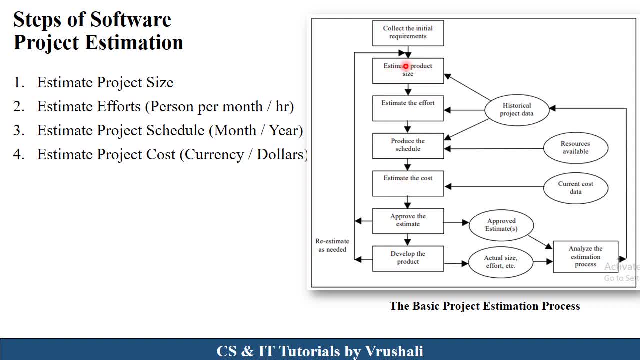 there are four main activity in software estimation. the first, to estimate complete product size, to estimate efforts, to produce the schedule of particular project and estimate the total cost of particular project. and after completing this four step, there is a approval estimation. and after that, after approval, actual development have started. so let discuss now all these four steps in detail. 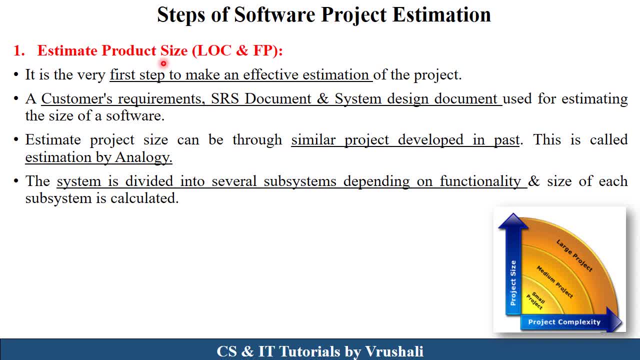 the first step in software project estimation is to estimate product size. see, there are some large project, some medium project and some small scale projects are available, right. so project manager, ensure that the complete project size according the customer requirements, then srs documents, system design documents. they analyze all those thing and decide the size of particular project. 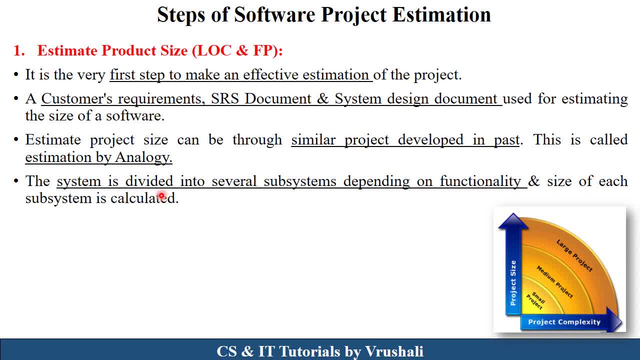 in planning phase there is a work breakdown structure. in work breakdown structure there are a work breakdown structure. your complete system is divided into the sub system and sub modules are there. so according to that, modules and functionality, project manager decide the size of particular project. or the next thing is how many lines are occurred in particular. 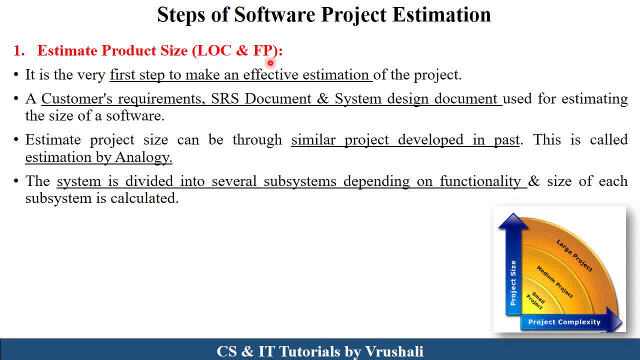 programming, that is lines of code, and functional point means how many functionality characteristics are included in particular project. according to that also, product size have decided and the next thing is: sometime what is needed to complete a particular item, mother report in project management. sometime what happen? the similar project have already developed in particular organization. 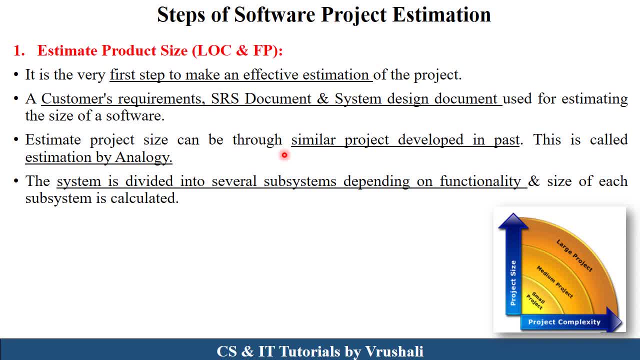 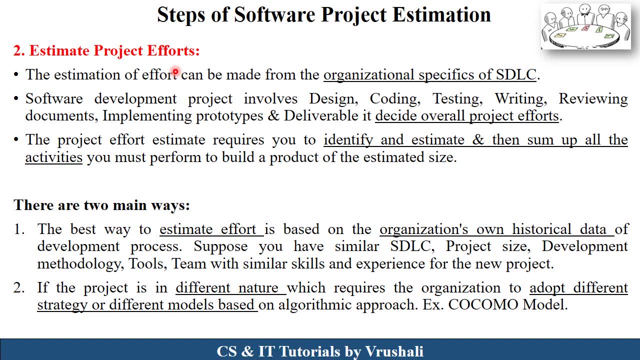 or in particular, company. so, project manager, as per the previous year project, they calculate size of particular project. this is called as estimation by analogy. now the next step is estimate project efforts, basically how many human resources are required for completing a particular project. this is called as estimate project efforts. see, suppose there is a small. 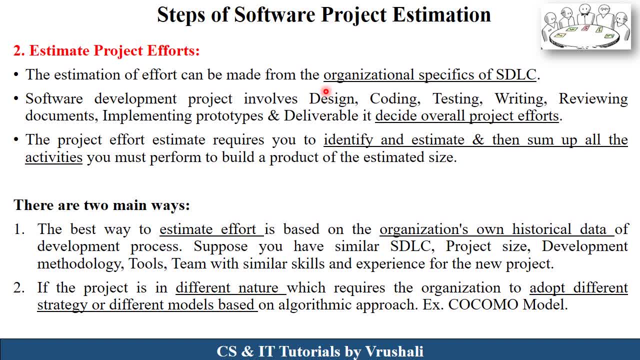 project cycle. so there is a different software development life cycle is used, but there is a large and complex project is there. so at that time in software development project there are design, coding, testing, then writing, reviewing documents, implementing prototype, then deliver a particular product. this all types of phases have included. so, according, 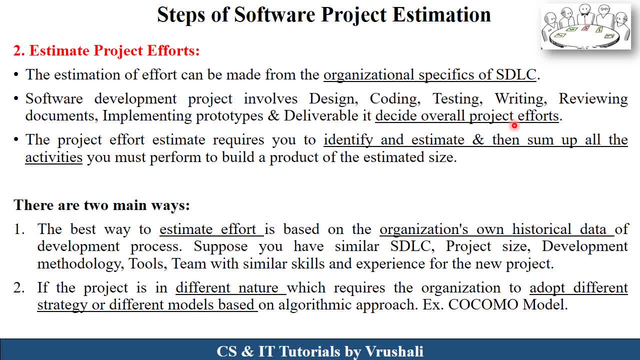 to that phases project manager decide how many human resources are required per over all project efforts. there are 2 main ways sometimes what happen? the similar type of project, similar type of software development life cycle and similar type of development methodology. tools teams are already developed in past project or some historical project, so at that time project manager analyze this. 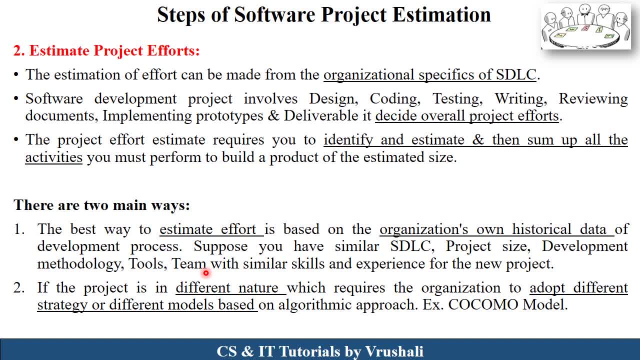 past project and give estimate project efforts according to that. and the next thing is: suppose particular project has already been analyzed. so after that in some historical project, there project is in different nature or new to the particular organization, so at that time project manager adopt different strategy and different models to calculate project efforts. for that 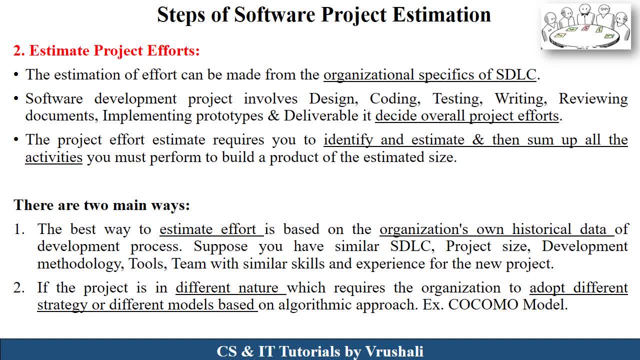 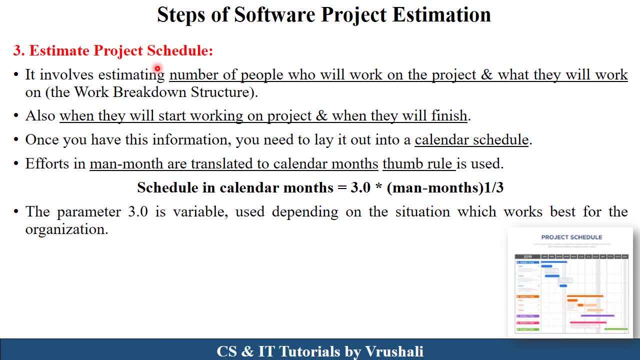 purpose kokomo model is used. we will discuss kokomo model in detail in next session. now the third step is estimate project schedule. so basically, project manager estimate that number of people who will work on particular project and what they will work. they also decide when the particular project have started and when particular project will finish. they 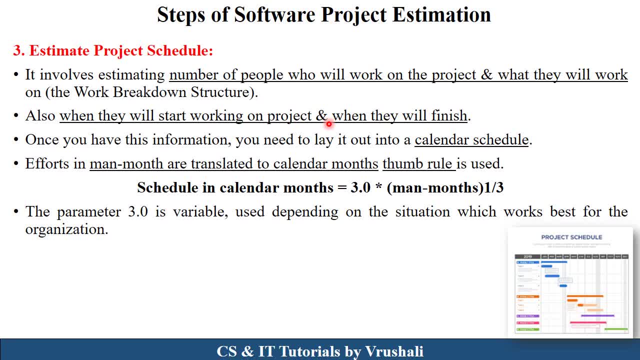 decide planning date, actual date, start date, end date of each and every activity in software development schedule. sometime, project manager also use term rule for calculating project schedule, that is, schedule in calendar months equal to 3.0 into how many human resources are required per month in particular project. 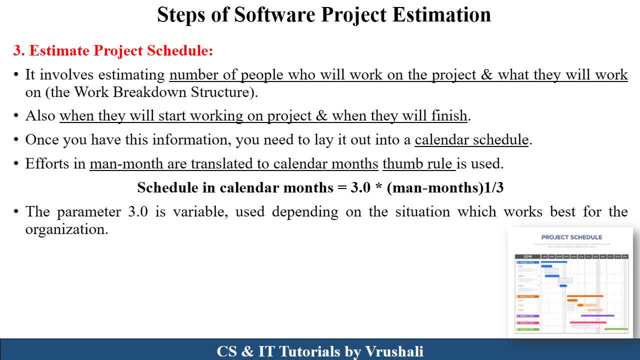 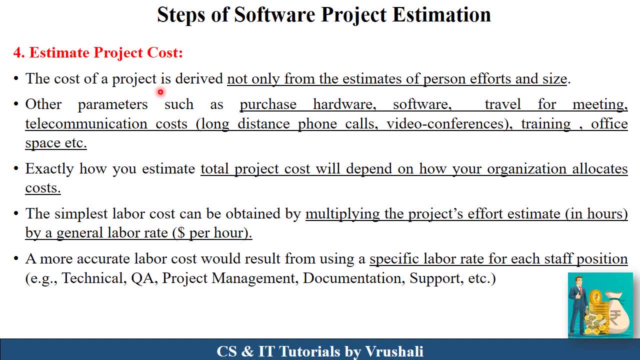 according to this. so this is a formula for calculating project schedule. now the last step is to estimate project cost. see, project cost is not only depend on how many human resources and what exactly size of particular project. the project cost also depend on how many hardware and software resources are purchased, then travel for meeting, then telecommunication. 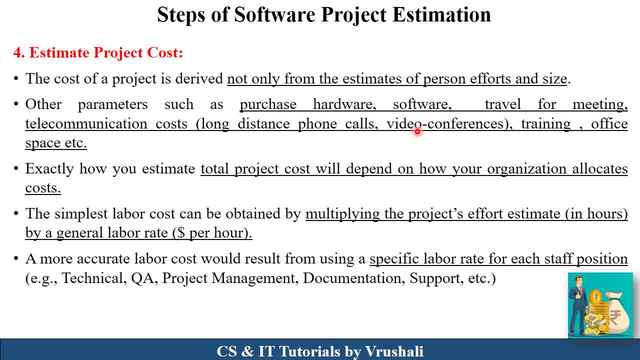 cost means sometime long distance phone call video conference are there in particular project, then training cost is there, then office space cost is there. so this: all factors are considered while estimating a project cost exactly. project manager estimate: total project cost will depend on how your organization allocate a particular cost and as per the thumb rule. 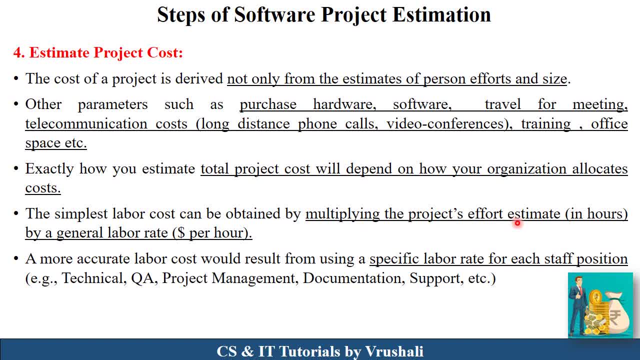 project cost have decided as per the project effort estimation in our means, human per human in our, how many cost is required. so according to that they calculate project cost. and also there is a salary division of each and every employee. so project cost also depend on technical person, quality assurance, project management documentation, supports. so by 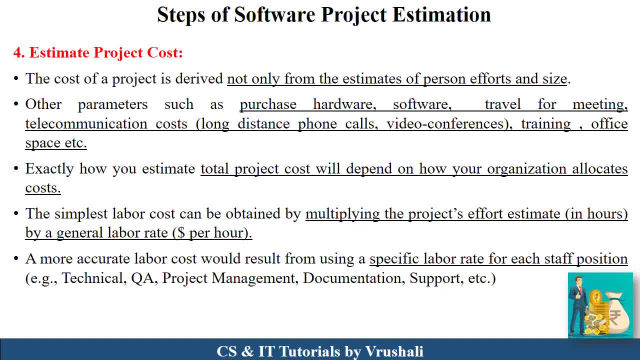 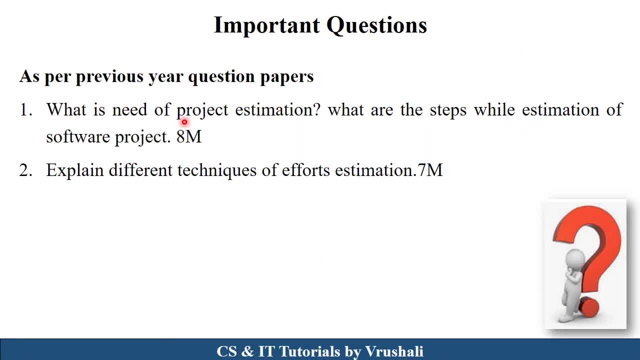 considering all these factors, project manager estimate the project cost and budget at early stage of project development. now these are the some important questions that have asked in previous year question paper, like: what is the need of project estimation and what are the steps while estimation of software project? sometime they ask, explain the steps while estimation of 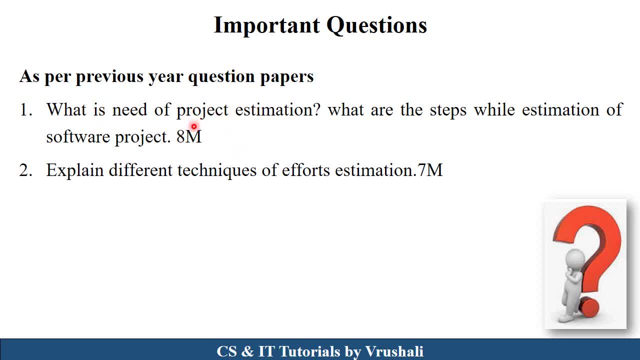 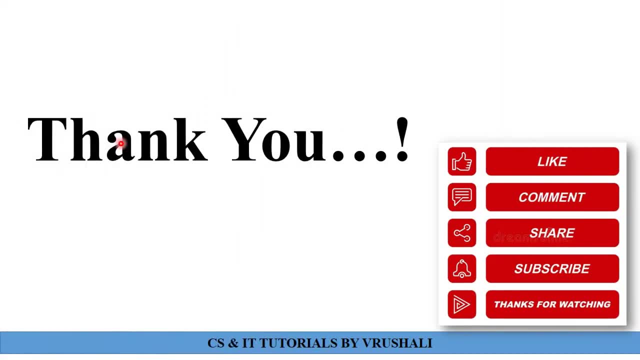 software project. so you have to prepare all these four steps in detail for eight marks and explain different techniques of effort estimation for seven marks. thank you, keep learning. 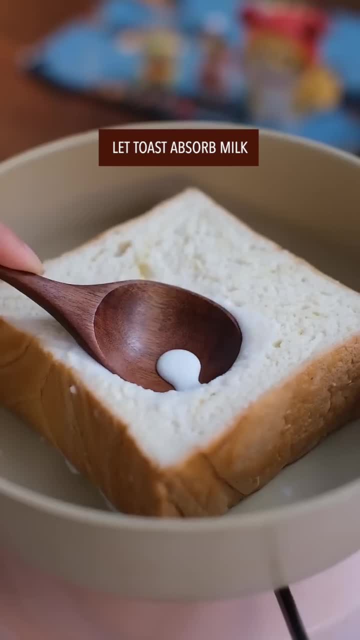 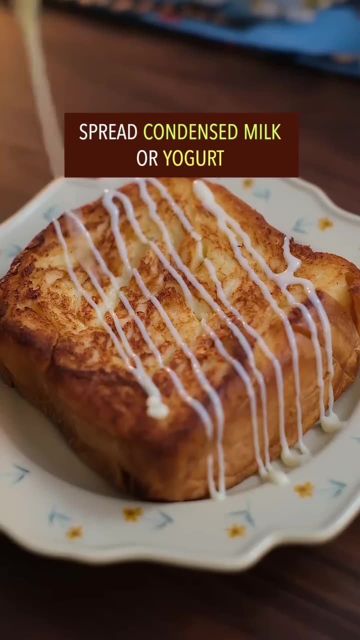 A thick piece of toast. Add whole milk, Let toast absorb it Evenly. spread melted butter Slowly move it around. Fry both sides on low heat until browned. Transfer to a plate Condensed milk or yogurt, Done and dusted.